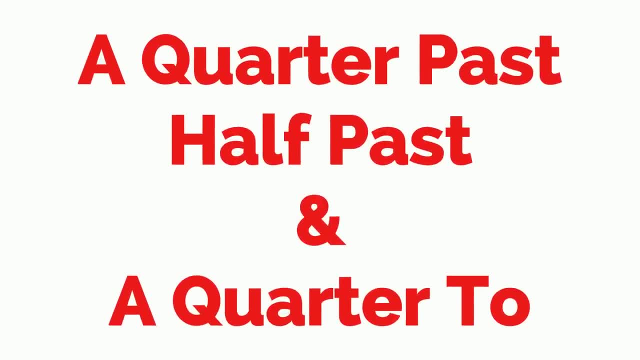 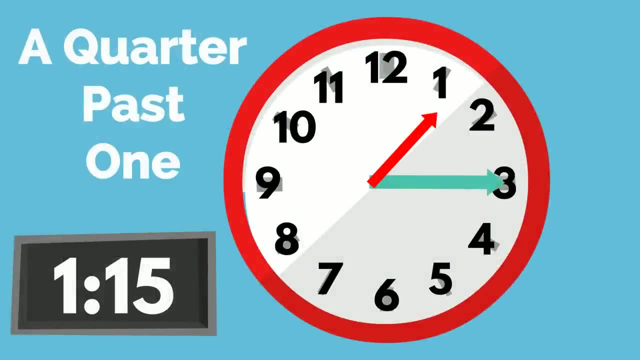 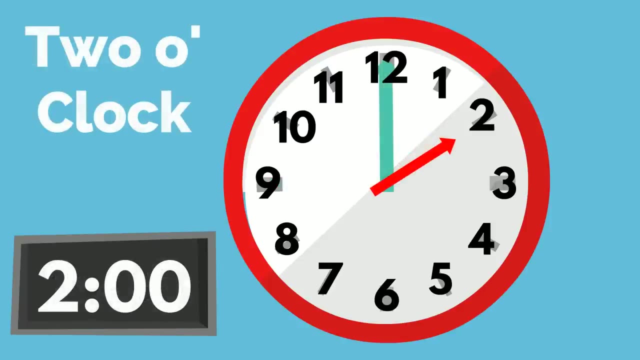 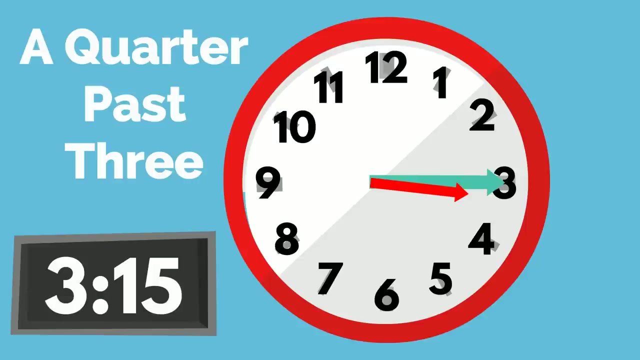 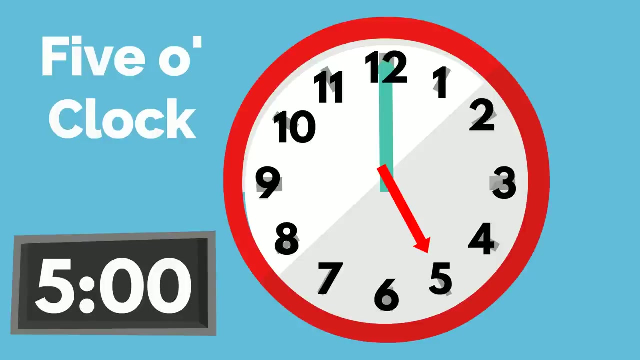 Let's tell time with: a quarter past, half past, and a quarter to A quarter past. three. half past three. a quarter to four, four o'clock. a quarter past four, half past four. a quarter to five, five o'clock. a quarter past five, half past five. a quarter to six, five o'clock. 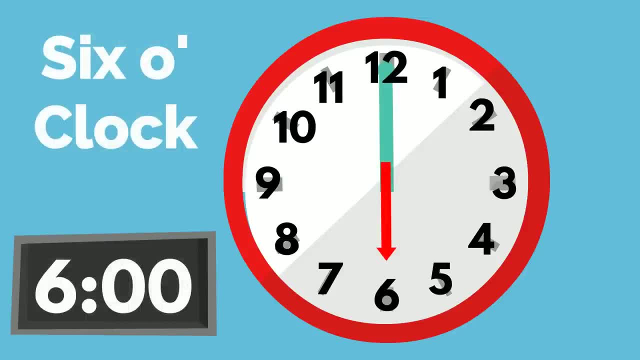 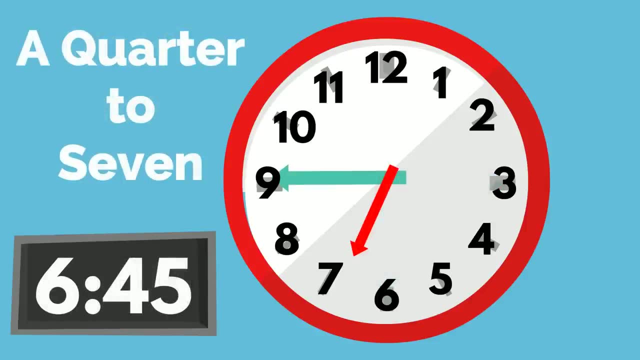 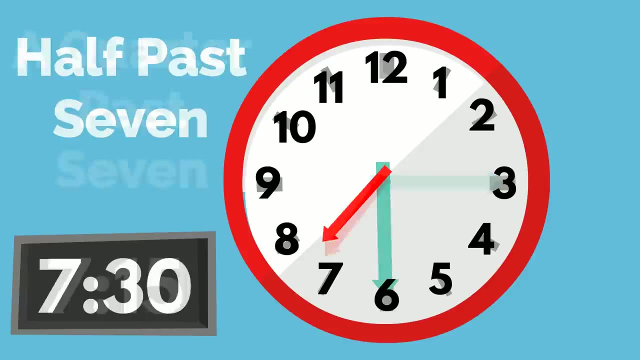 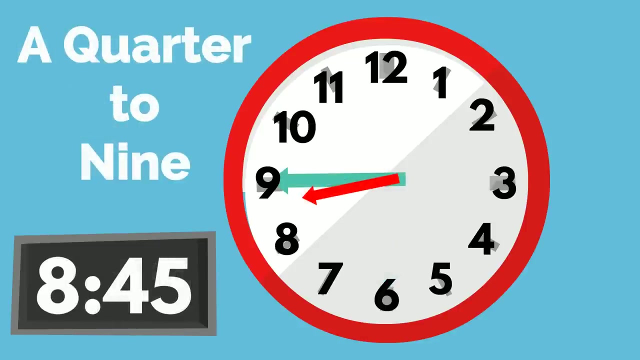 Six o'clock, a quarter past six, half past six, a quarter to seven, seven o'clock a quarter past seven, half past seven. a quarter to eight, eight o'clock, a quarter past eight, half past eight a quarter to nine, nine o'clock a quarter past nine, half past nine, a quarter to ten, ten o'clock a quarter past ten, half past ten, a quarter to eleven, eleven o'clock. 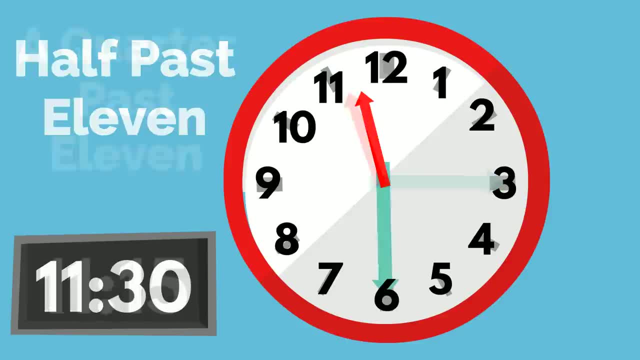 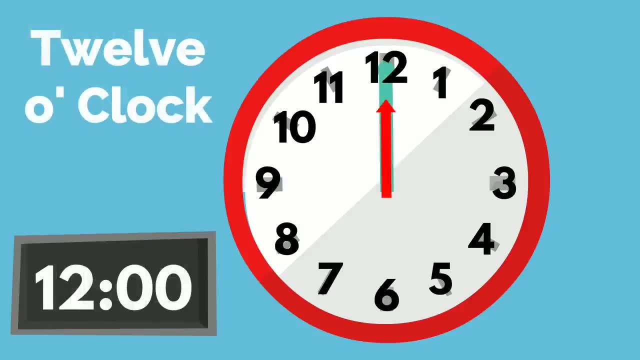 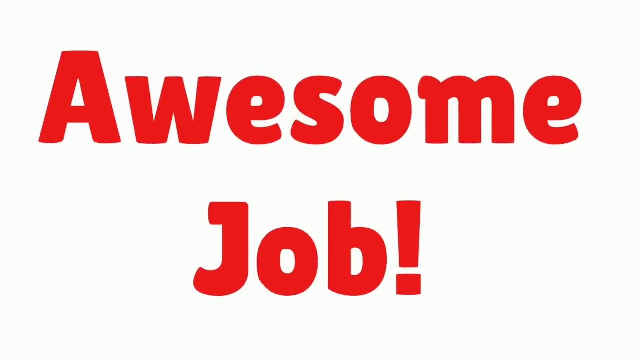 a quarter past eleven. a quarter past eleven, half past eleven. a quarter to twelve. twelve o'clock, a quarter past twelve, half past twelve, a quarter to one, one o'clock. Awesome job. Remember to like, subscribe and comment below. 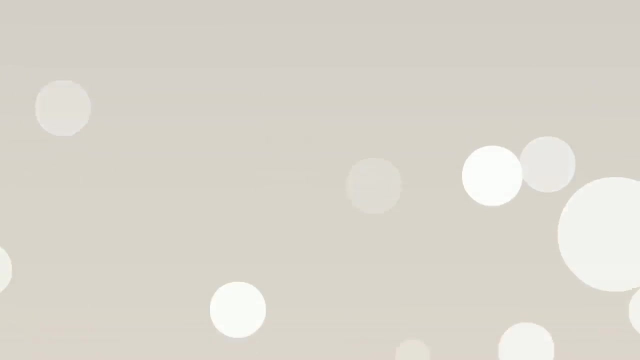 Thanks for watching. Don't forget to turn on your notifications so you don't miss out on any of our new videos. Thanks,